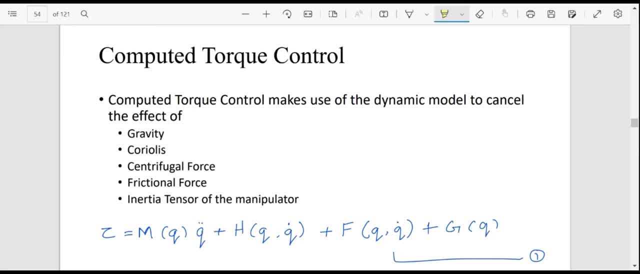 In this video, we are going to see about computer talk control. Generally, when we discuss control schemes, we will always discuss one degree of freedom schemes. That is for ease of understanding. But practically, we have n degree of freedom schemes or n degree of freedom systems. So, one degree of freedom schemes fall under SISO, single input and single output. 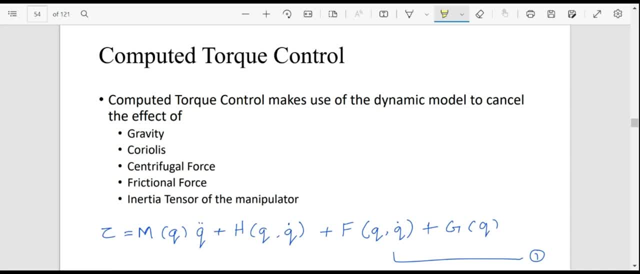 But practically, we have multiple input and multiple output. When we have to solve problems with multiple input and multiple output, we have to analyze all the dynamics of the system. 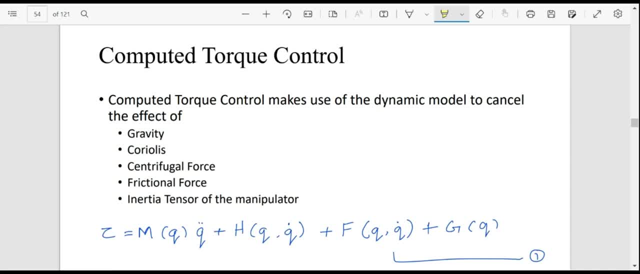 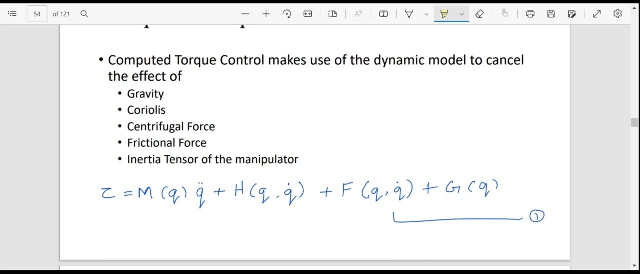 So, this computer talk control makes use of the dynamic model to cancel the effect of gravity, Coriolis, centrifugal force, frictional force, inertia tensor of the manipulator. The controller discussed here employs the computer talk control law to modify the system and effectively decouple 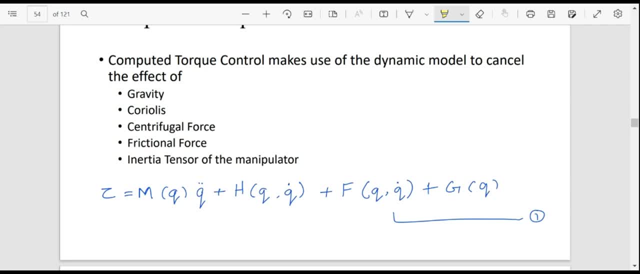 and linearize it. The non-linear dynamic model of the n degree of freedom manipulator based on the rigid body dynamics gives the n cross 1 vector of joint talks. This is that n cross 1 vector of joint talks. 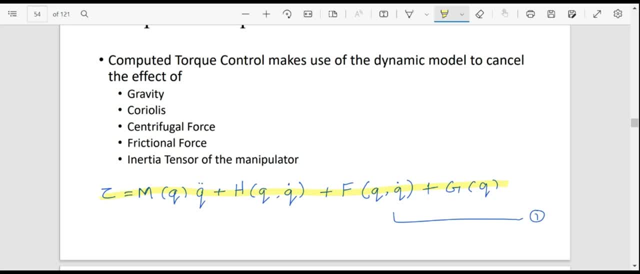 So, this n cross 1 vector of joint talk we have n cross n inertia matrix, this is the n cross n inertia and this is n cross 1 vector of centrifugal and Coriolis talks. This is the gravity talks again this is n cross 1 vector and these all adds up to the other forces. So, what is the only one texture bulk that the hopefully the most remarkable project will be. 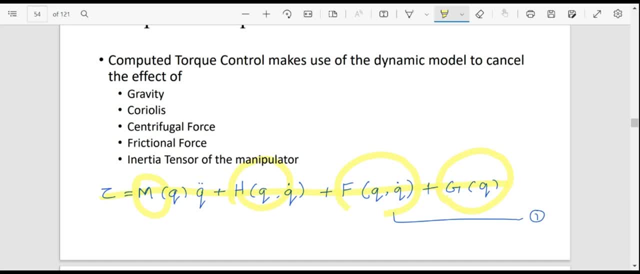 which are like overall contribution of friction and other non-rigid body effects. 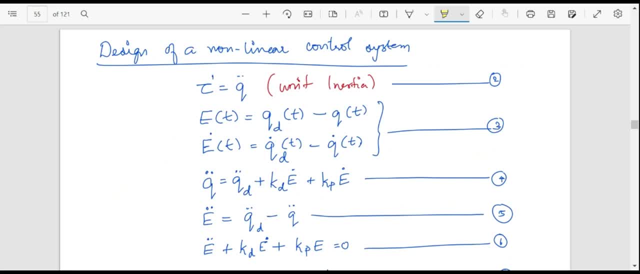 So, while designing a non-linear control system, we have to understand that similar to the previous partition control schemes, here also we have partitioned the control scheme into two, a servo-based portion and a model-based portion. So, the controller based on this complicated model provides better trajectory tracking performance than linear controllers do. The reason behind this is this controller, which is designed now, uses computer torque control to modify the system and effectively decouple and linearize it. First, let us calculate the servo-based portion. So, we have a servo-based portion and a model-based portion. So, the controller based 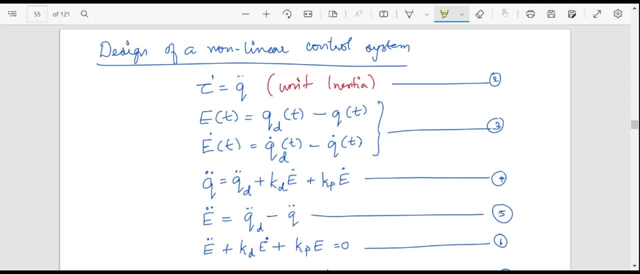 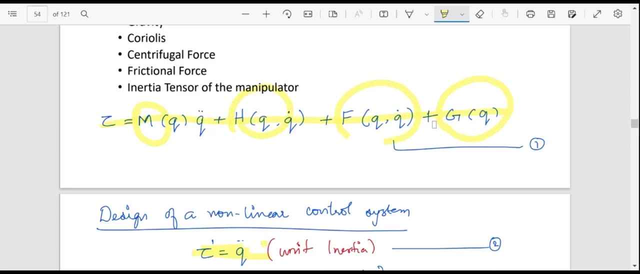 portion, to equate the system assuming unit inertia. To calculate the servo-based portion, we equate the system assuming unit inertia. We have done this previously in the position control system also. The torque, the frictional force contribution and this h factor, 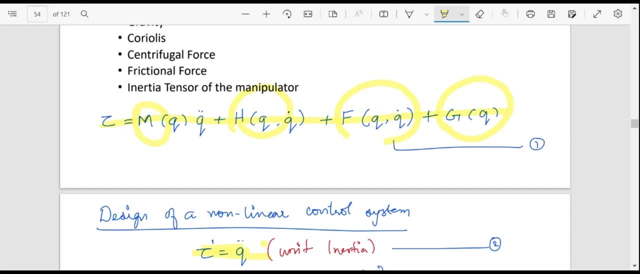 which is the centrifugal and coriolis torque, these are all remain zero. 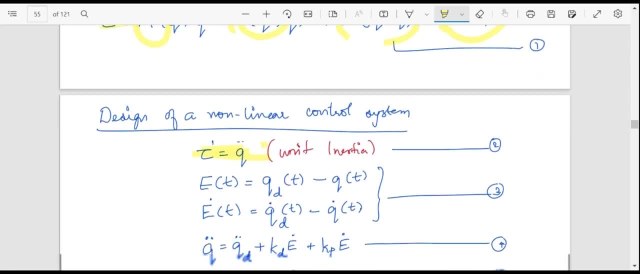 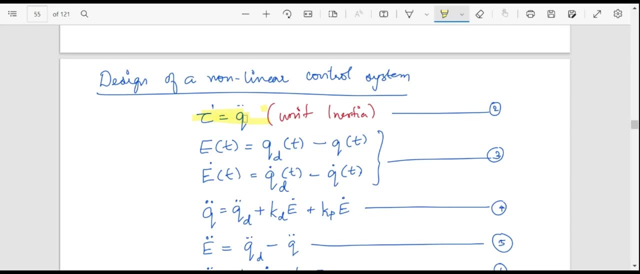 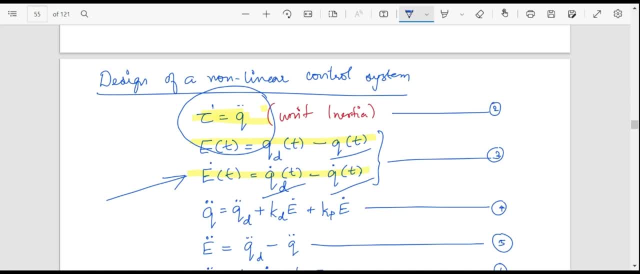 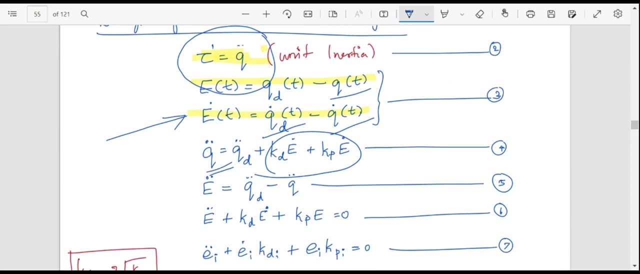 So, to calculate the error dynamics of the system, let us assume that the actual acceleration is equal to desired acceleration plus the controller coefficients. So, here K d, 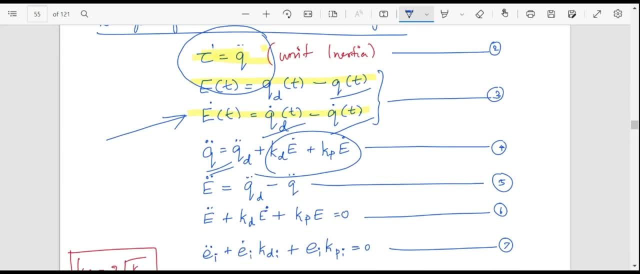 we know that what is K d. K d is the velocity gains of the joint acceleration. 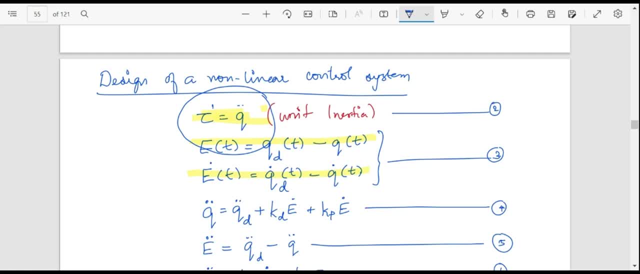 Okay. So, here E of t is equal to Q d of t minus Q of t is the P. error of position. This is the servo error for velocity and respectively this q d of t 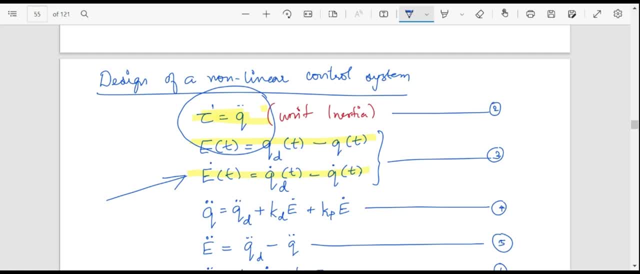 is the desired joint position and q of t is the actual joint position. 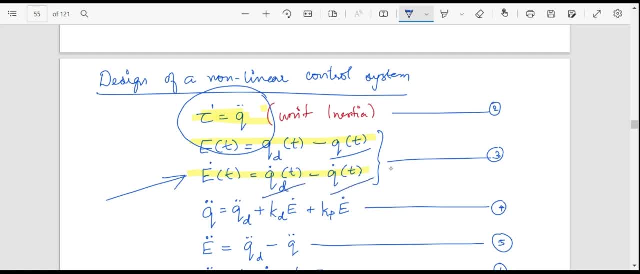 This is desired joint velocity, this is actual joint velocity. 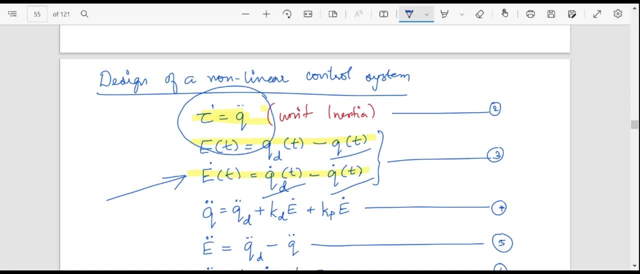 So, then we are going to calculate the error dynamics of this system. So, to calculate the error dynamics of the system, let us assume that the actual acceleration is equal to desired 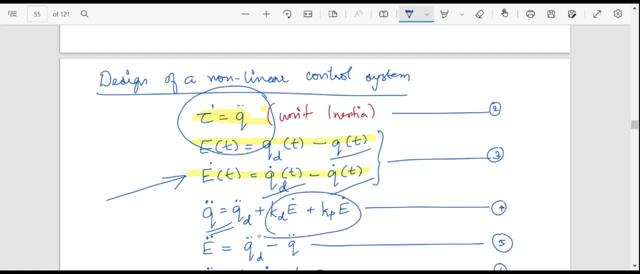 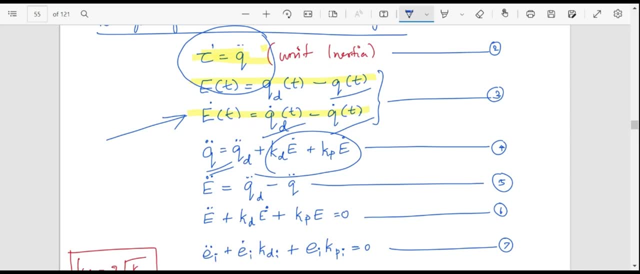 actual acceleration plus the controller coefficients. So, here k d, we know that what is k d? k d is the k d is the k d is the velocity gains of velocity gains. Here we know k d, k d is the velocity gain and k p is the 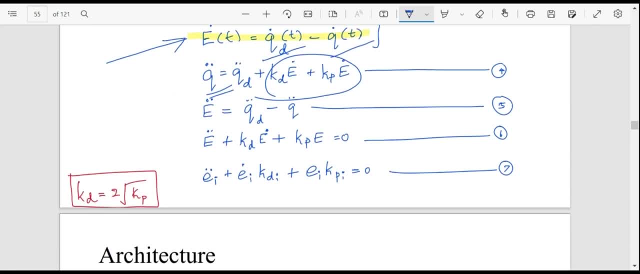 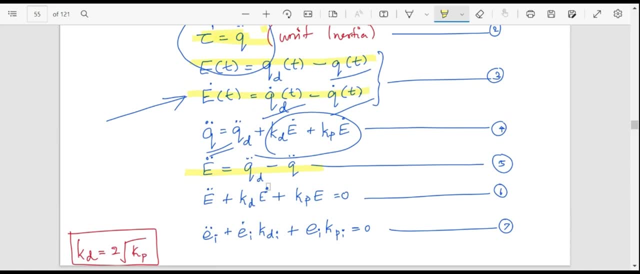 positional gain. So, when we calculate this, this acceleration error helps in deriving the error dynamics. So, when we calculate this, this acceleration error helps in deriving the which is given as equation number 6. So, if you look at the error dynamics of this system, this is a closed loop system and this error dynamics is specified by a second order linear error equation. And also, please understand that this equation number 6 is a vector equation 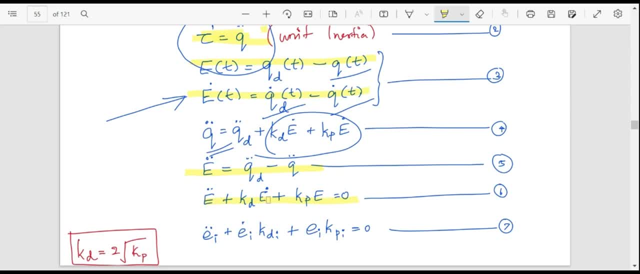 and it can be decoupled on one condition if this k p and k d are diagonal matrices with constant gain. So, absolute 해� Итак, 우리는 단atten dez. Decoupling will help us in working with individual joints as we are dealing with 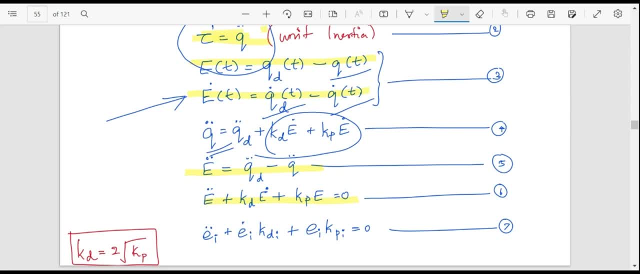 multiple joints since we have n degrees of freedom systems. 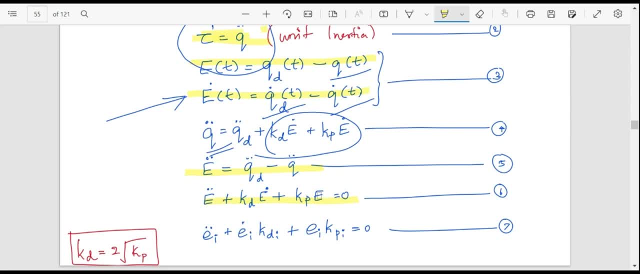 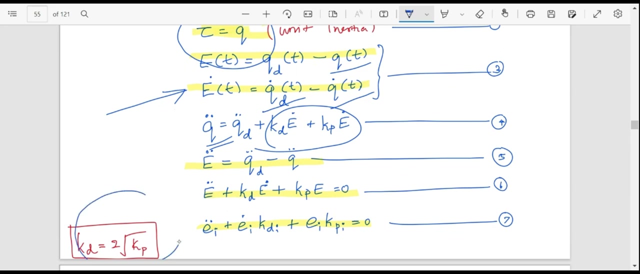 If you write the error equation on a joint by joint basis, we will get for the ith joint, this error equation, the same bay equation 6 can be read it and ask the error equation 7 here k d, k d 1 gegenüberniθ And we know that Kdi is the velocity gain of joint I and Kpi is the positional gain of joint I. We have already seen that for a robot manipulator the joint should be critically damped hence this condition must be satisfied, this condition must be satisfied where Kd that is the velocity gain is twice the square root of positional gain. If you maintain this our manipulator or the joint would be critically damped. There are few limitations in this system. Limitation number one the system is complex. 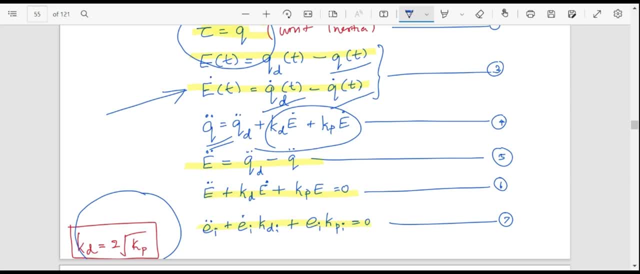 So we do not assume everything in this system. We take everything in this system into consideration. So things are complex. 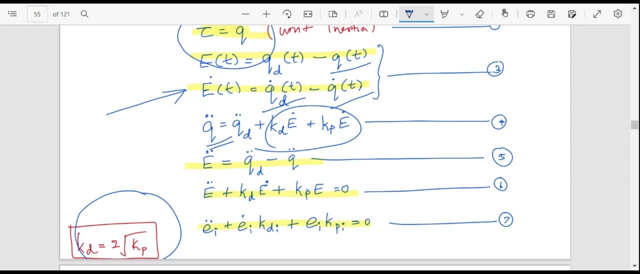 So any error which occur on any of the parameters. meters can affect the system point number two our limitation number two is this is computationally 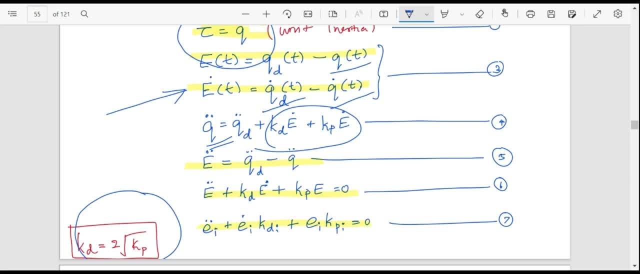 expensive we need we need computers which are very fast and for slower computers it takes time for calculation okay so to avoid this to avoid this we can follow various methods